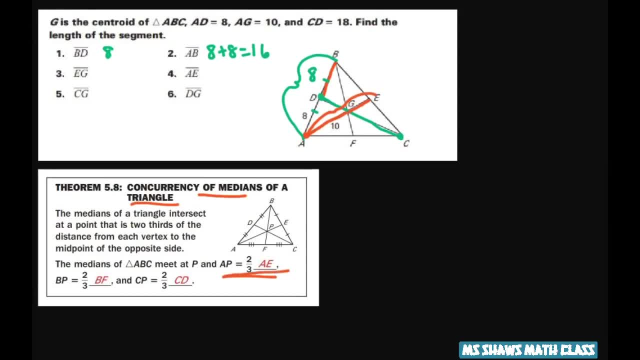 And that's basically what this is. So AG is two-thirds of AE. So AG is 10 equals two-thirds of AE, And we're going to multiply both sides of the equation by the reciprocal of two-thirds, which is three-halves. 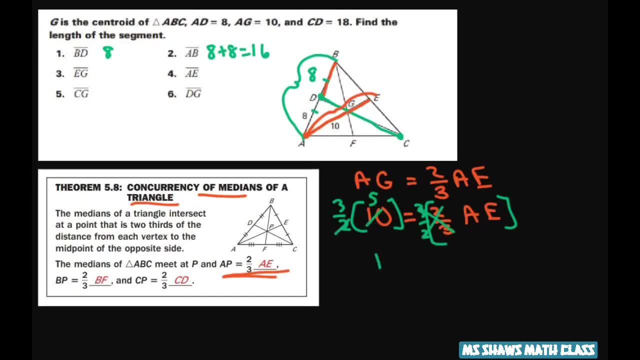 So two goes into 10, 5.. So that's going to be 15 equals the length of AE, So that's 15.. So to get GE or EG, we just take our 15 minus 10 equals 5.. 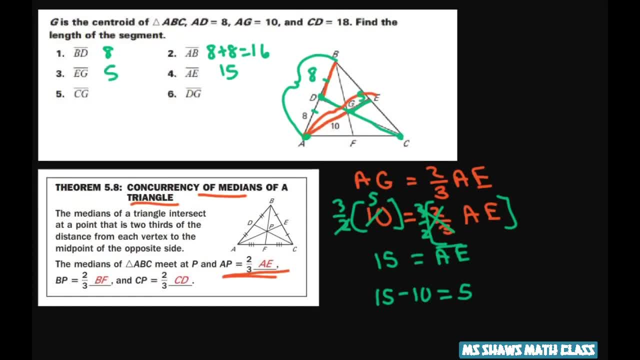 And so this would be 5.. Remember, the length from the vertex to the centroid is two-thirds of the total length, And the 5,, therefore, is one-third of the total length of 15.. Okay, CG. Okay, so let's erase this. 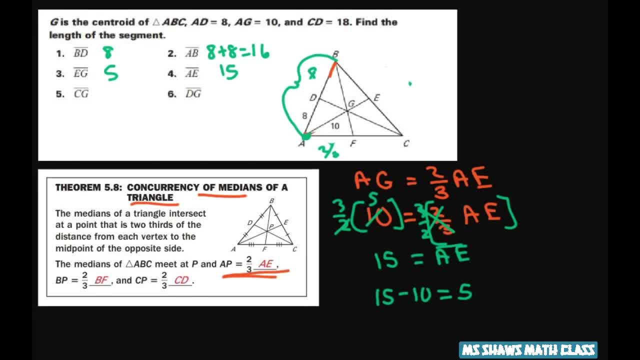 CG is this part, So we need to find CD. It's not marked, It's 18.. So we know that CG is two-thirds of the total length, which is CD. So CG is going to equal. I'm going to keep writing G first. 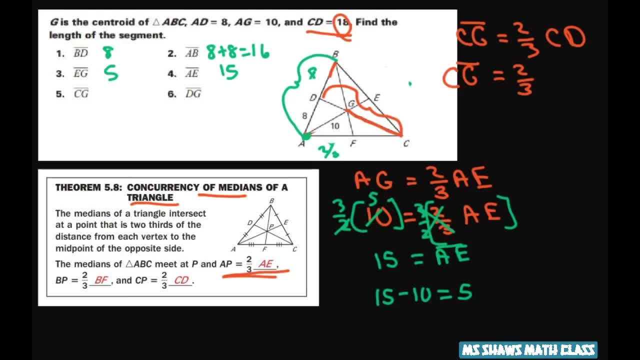 It's two-thirds of 18.. So 3 goes into 18 six times, And 6 times 2 is 12.. Therefore, DG is just going to be 18 minus 12, which is 6.. And again. 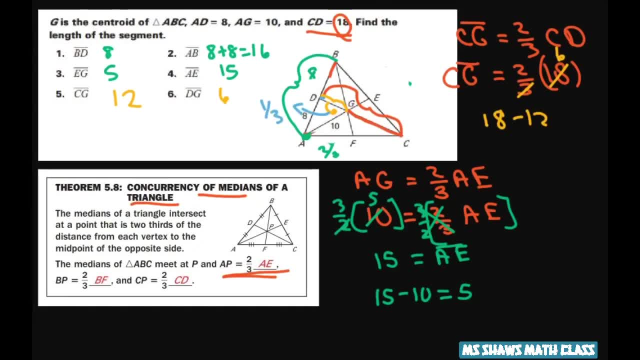 this is the one-third part, because it's going to the midpoint, And the CG, which was 12, is the two-thirds part, And that's it. Thank you, Have a nice day. Bye-bye.